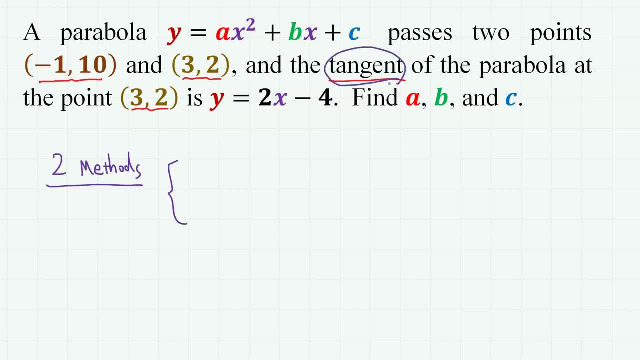 And I will present you two methods. When dealing with tangents, the most obvious way to approach is, of course, using the mighty calculus, But here the given function is quadratic function, so we can solve this problem without using calculus. Therefore, I am going to solve this. 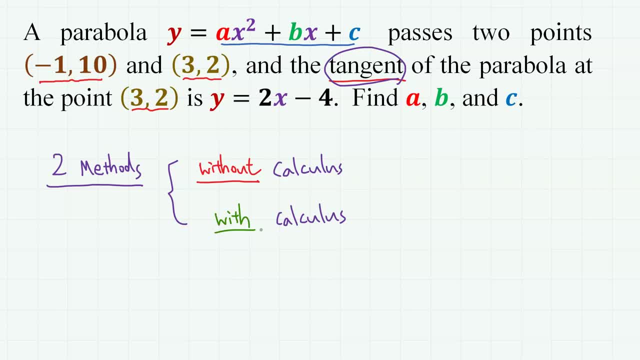 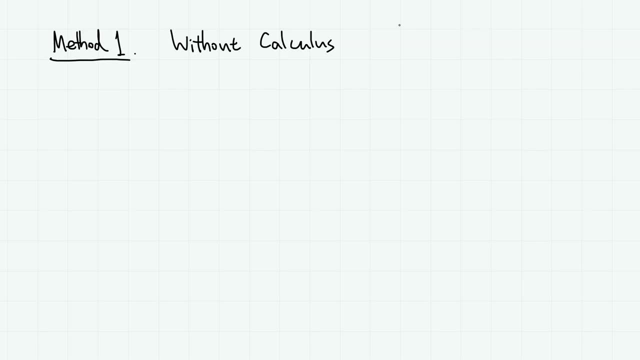 problem first without calculus. Then I will present you the method with calculus. All right, so the first method without calculus. Instead we will use the relation between quadratic function and the roots of quadratic equation. First, the parabola passes points minus 1 comma 10. and 3 comma 2.. And then the tangent of the parabola passes two points minus 1 comma 2 and 3 comma 2.. And then the tangent of the parabola passes points minus 1 comma 2 and 3 comma 2.. So 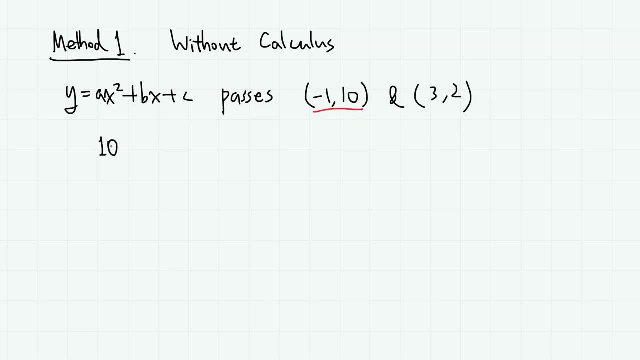 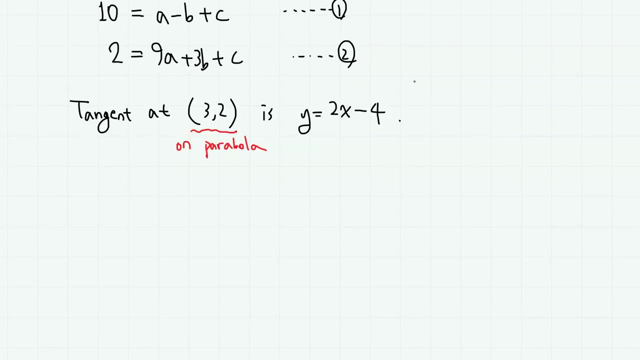 3,2.. So, using this point, we have 10 equals a minus b plus c, And using this point, we have 2 equals 9a plus 3b plus c. So we have two equations. Next, we use the tangent condition, Since y equals. 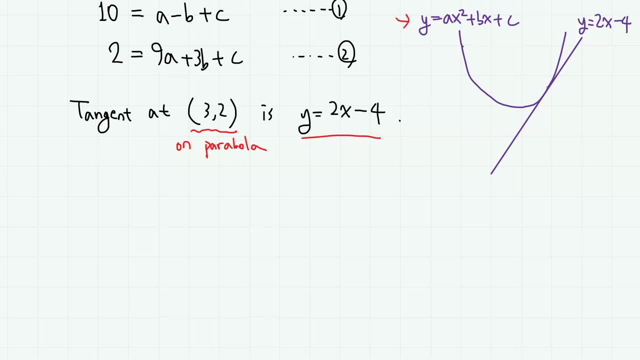 2x minus 4 is a tangent line to this parabola. two graphs only have one intersection point. This means that this quadratic equation, ax squared plus bx plus c equals 2x minus 4, has repeated root right here, which is x equals 3, as given in the problem. So by rearranging this, 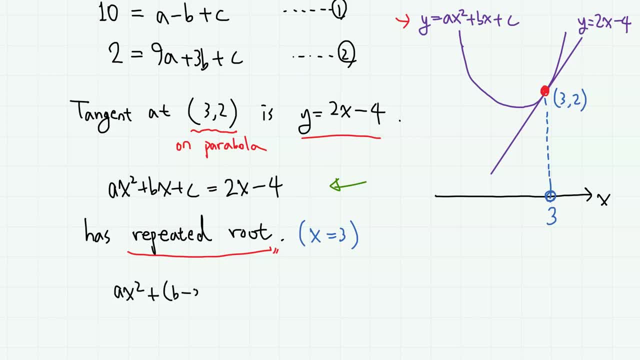 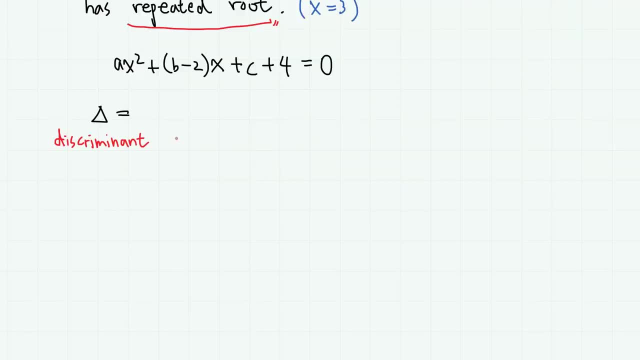 equation we have ax squared plus b minus 2x plus c plus 4 equals 0. In order to have repeated root, the discriminant of this equation must be equal to 0.. So we have b minus 2 squared minus 4a times c plus 4 as the discriminant, and this must be 0.. 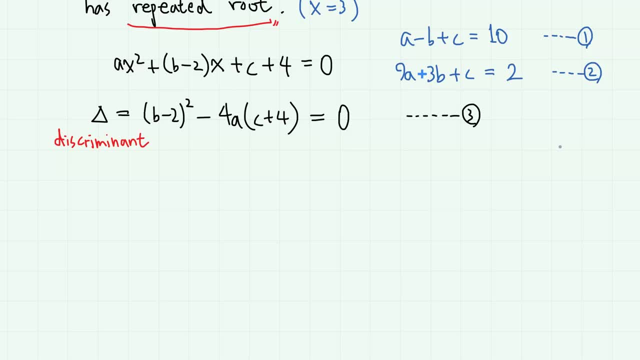 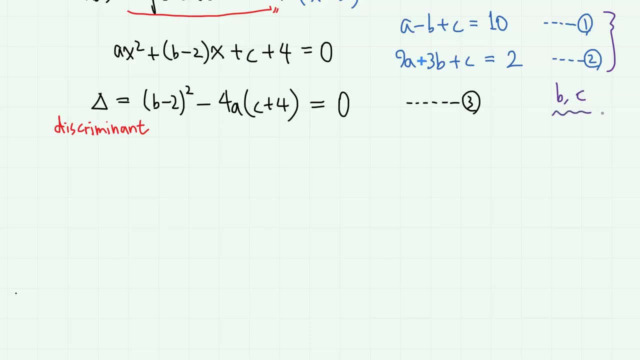 And this is our third equation. So now we have three equations with three unknowns. Now how can we solve them? From these two equations we can express b and c in terms of a. From equation 2 minus equation 1, c is eliminated and we get 8a plus 4b, equals. 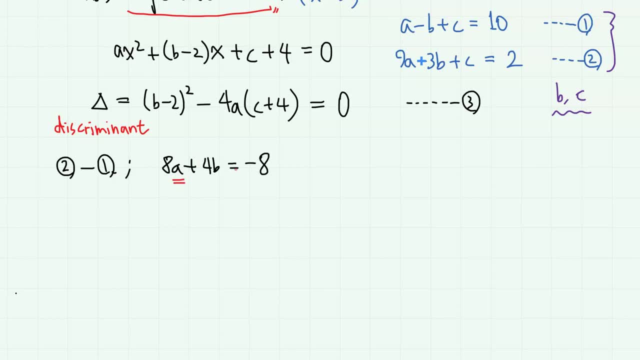 minus 4a. So we have b minus 2, squared minus 4a, times c plus 4 as the discriminant, and this must be minus 8.. Treating a as the constant and solving for b, we get b equals minus 2a minus 2.. 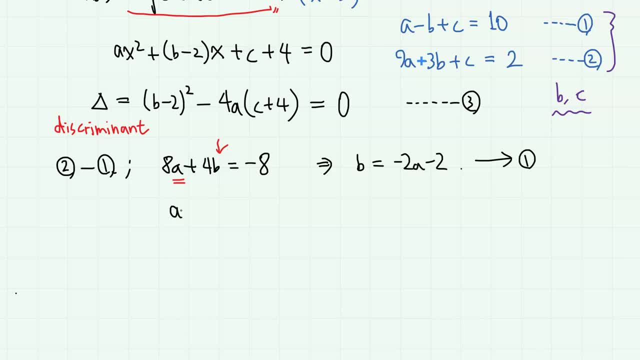 Substituting this expression in equation 1, we have a minus minus 2a minus 2, as b plus c equals 10. So, again solving for c, we obtain c equals minus 3a plus 8.. Substituting these values in 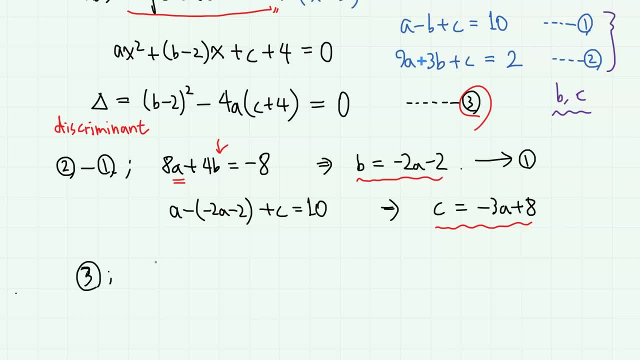 equation 3, we have b minus 2, squared minus 4a plus 4a. So we have b minus 2, squared minus 4a is minus 2a minus 4. squared minus 4a times and c plus 4 is minus 3a plus 12 equals 0.. 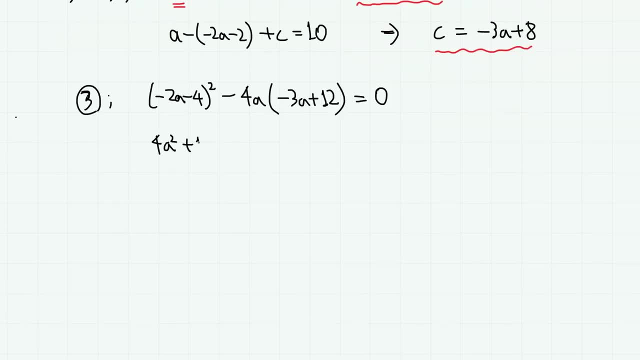 So we have 4a squared plus 16a plus 16 plus 12a squared minus 48a equals 0.. Therefore, we have 16a squared minus 32a plus 16 equals 0.. So we have 16a squared minus 32a plus 16 equals 0.. So we have. 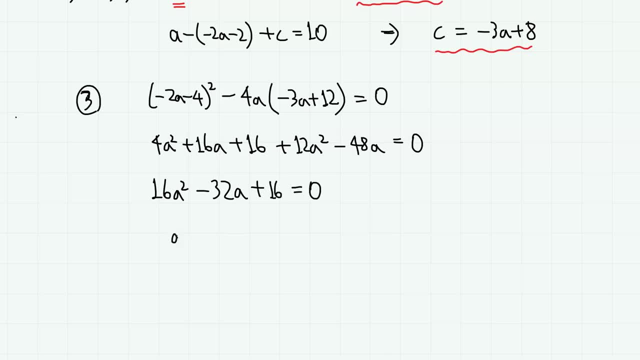 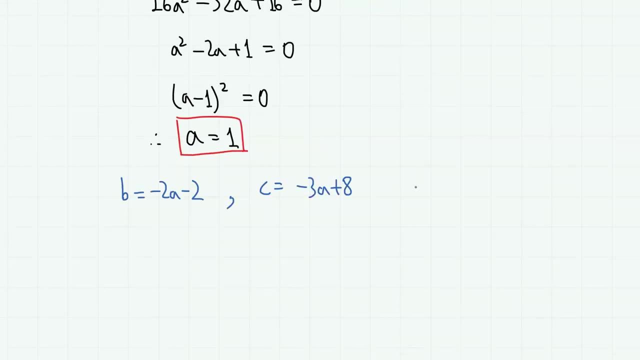 16a squared minus 32a plus 16 equals 0.. So we have 16a squared minus 32a plus 16 equals 0.. And if we divide both sides with 16, we have a squared minus 2a plus 1 equals 0, which is a minus 1 squared equals 0.. Therefore we have a equals 1.. And we have already solved b and c in terms of a, So using these, we obtain b equals minus 4 and c equals 5.. And these are the answers. 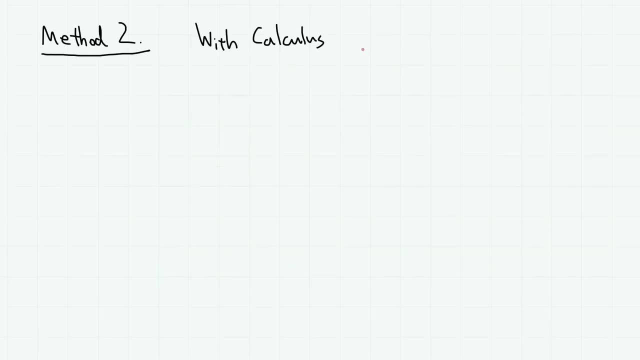 And the second method. The faster and more general way to solve this kind of problem is, of course, calculus. First, since the parabola passes point minus 1 comma 10 and 3 comma 2, we have a minus b plus c equals 10, and 9a minus 3b plus c equals 2.. So these two equations are the 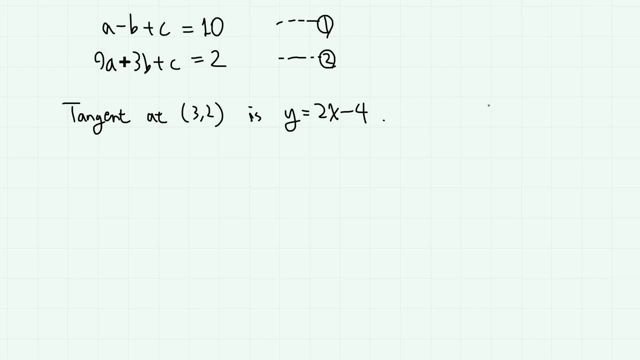 same as in the first method. Now we use the calculus for the tangent condition. From this equation we have y prime the derivative as 2ax plus b. Since the tangent at point 3,2 on the parabola is y equals 2x minus 4, from the slope condition, the value of the derivative at x equals 3 must be.